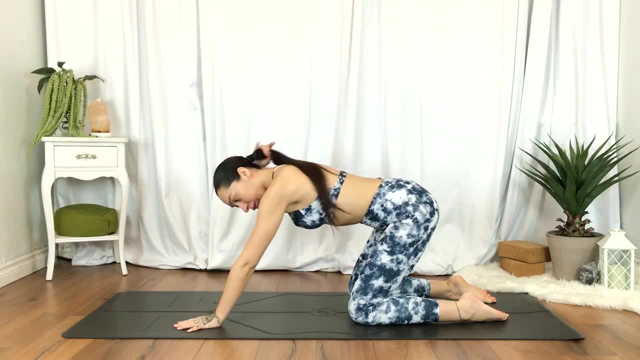 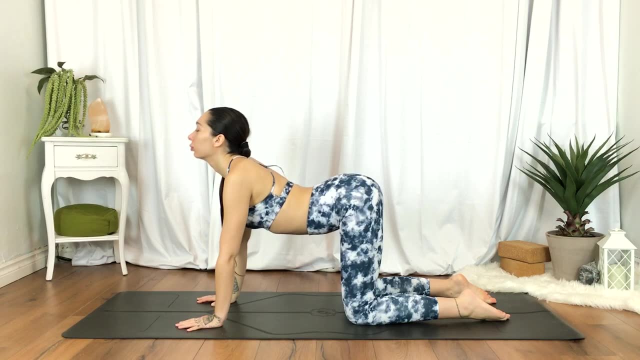 free to modify when and where needed. Let's begin in tabletop: Wrists under shoulders, knees under hips. Inhale, dropping the belly Gaze up for cow pose, Exhale, rounding through the spine Gaze down for cat. Continue sinking breath with movement going at your own pace. 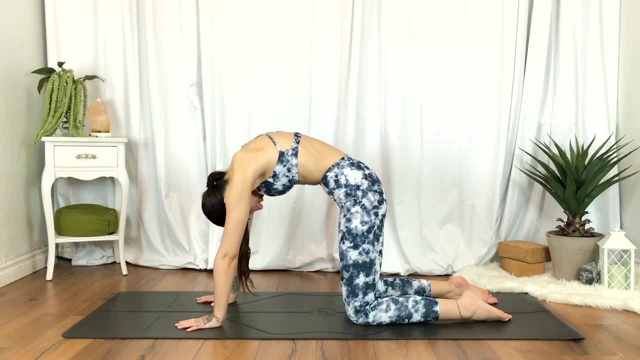 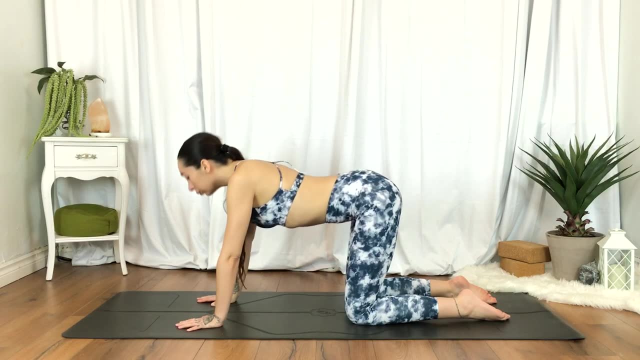 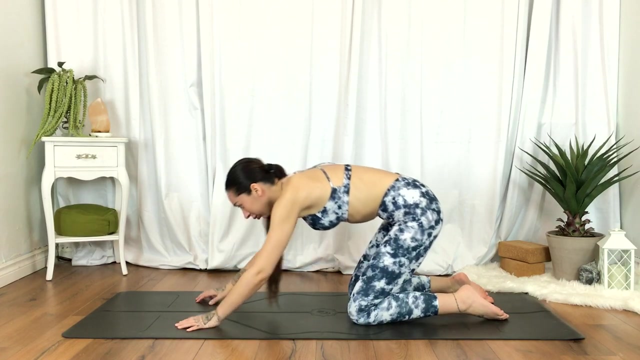 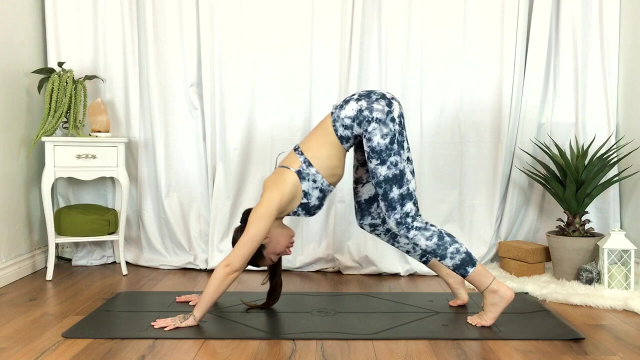 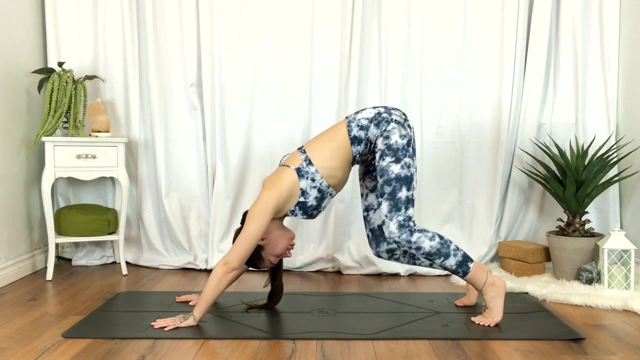 And when you're ready, we'll tuck the toes, sending the hips up for down dog Walking it out here. bend the hips, Bending one knee, bend the other, Maybe rocking the hips side to side. No worries about your alignment or what it looks like here, Just feel out the pose. 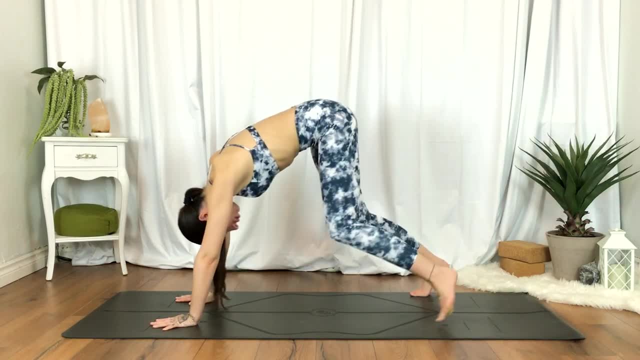 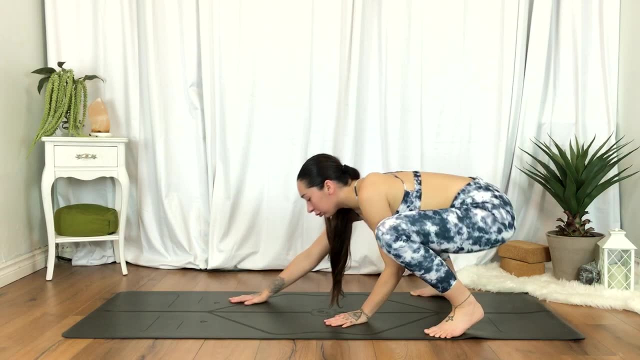 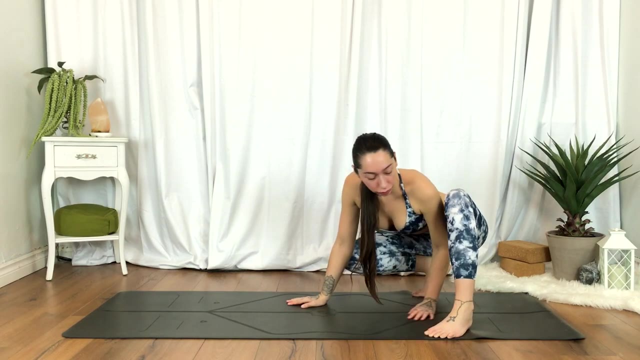 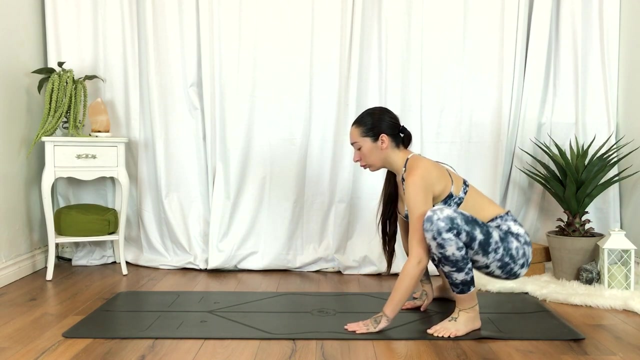 And then we'll start to take the feet mat with distance, While walking your hands towards your feet, Gentle sway, as you lower the hips, coming into Molossana, squat, Elbows to the inside of the knees, hands in prayer, Using your thumbs to lift your 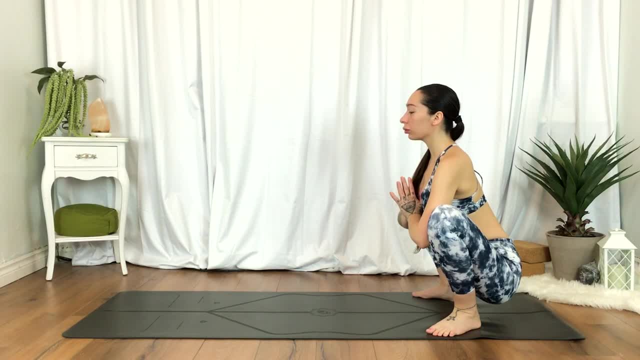 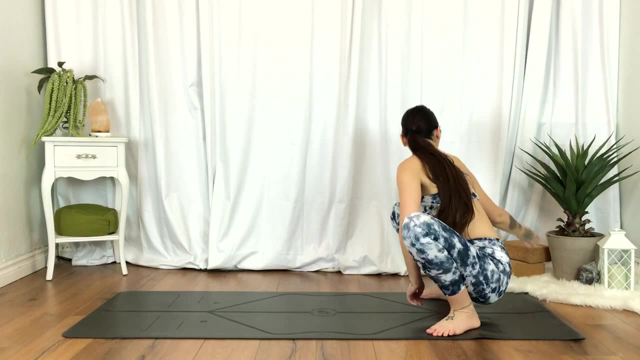 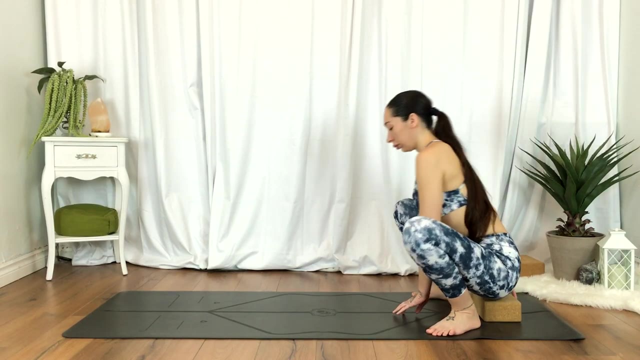 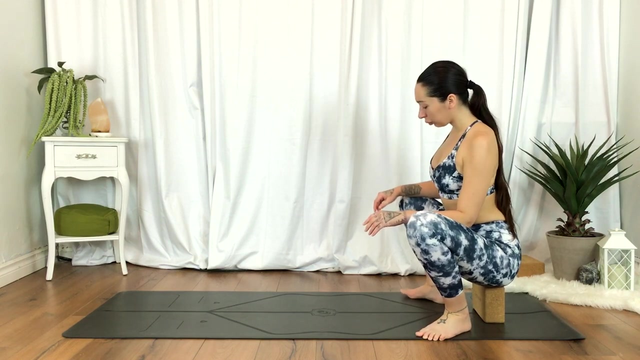 sternum lengthen through the spine. Now, if this is feeling intense, cry or like this. Hence, no worries. go ahead and sit on a block, or even a stool or stacked pillows as high as you need. Use your forearms or your hands to guide the knees open. 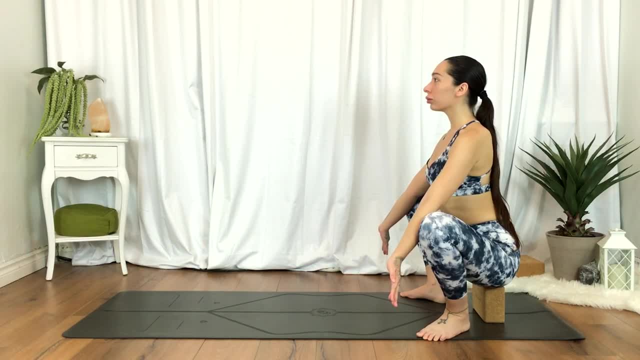 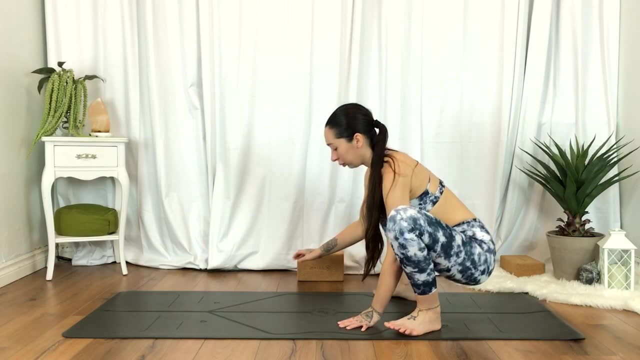 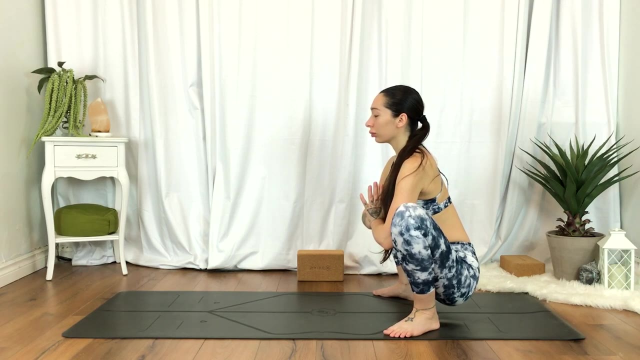 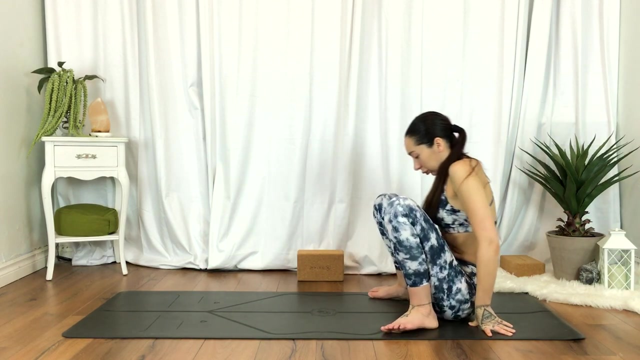 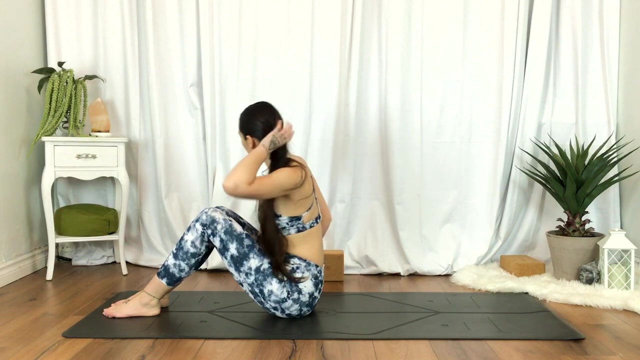 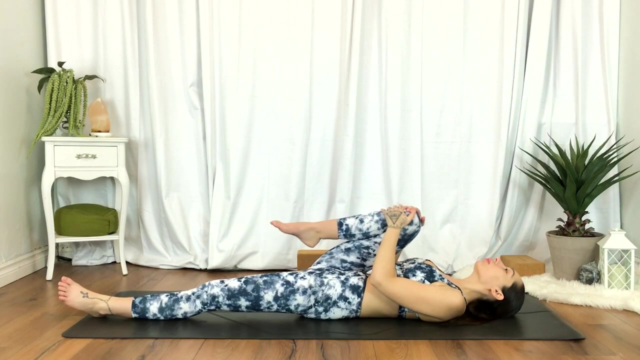 Don't force them, just guiding, naturally, Drawing the breath into the belly wherever you are. Exhale, softening the belly And we'll gently release. Come to your knees, Come to your back, Hugging the right knee towards the chest, as close as you can get it. 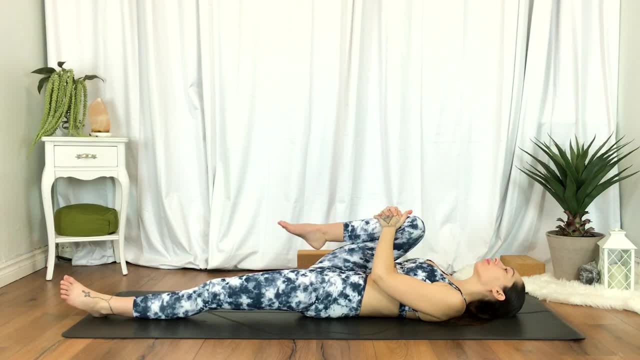 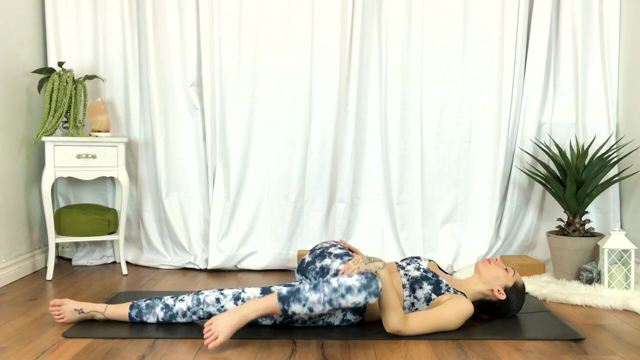 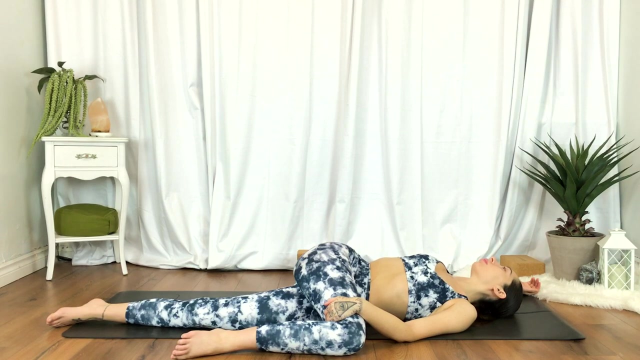 And we'll draw the breath into the belly As you exhale, softening the belly, And now the other foot. Think as if you are Cheeseful's cousin or dog. Go ahead and relax here. Just a few more breaths. For the next one. just breath in with your touch On your next exhale. Go ahead and cross the right knee over towards your left. Back stays flat on the mat for a supine twist Option to place as many pillows underneath the knee- as many pillows must fit. If you find a forme, flip it over. Leave an opening at the ankle, Keep the rocks until the skin is narrow. Step 4. Often that helps keep your body in the right position. If you do this- dry for wit to the pain- the body feels less muscle as you finish's the 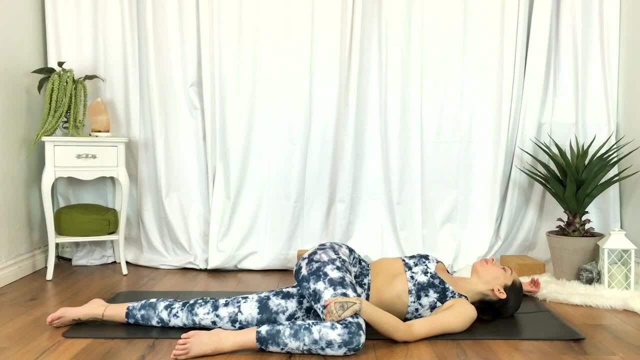 Later on, keep the body twice as convenient as you need. You can even place a pillow or folded blanket underneath the right shoulder for less of a twist, Observing the body and noticing where you're tensing up, If so, drawing the breath into that area As you exhale completely. 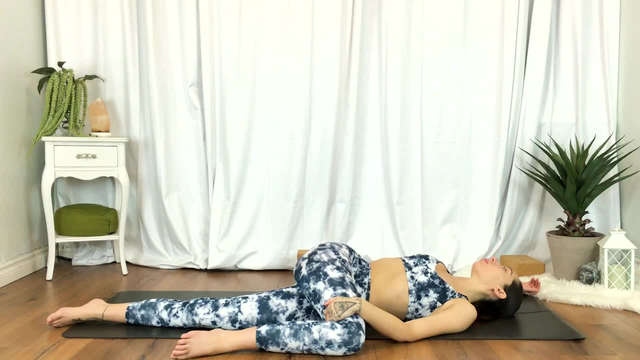 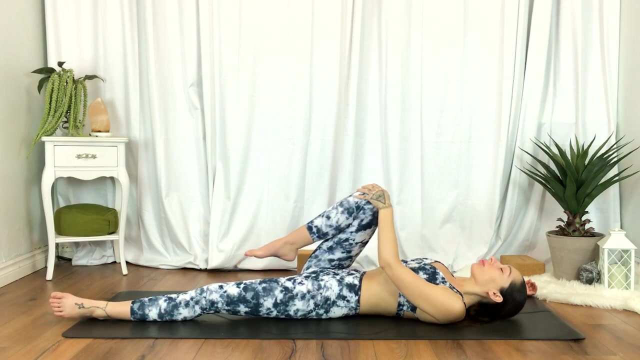 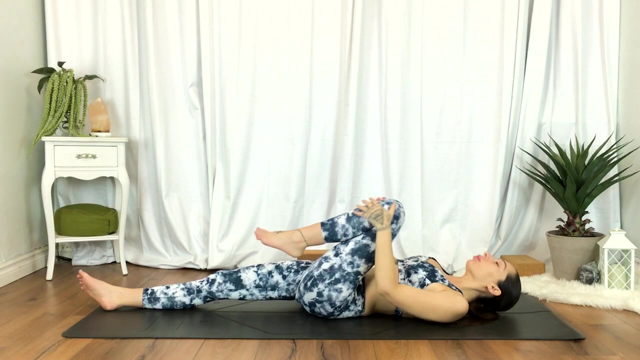 surrender. even if it's just for a moment, We'll inhale release, Switching sides, Hugging the left knee towards the chest as close as you can comfortably get it And just taking a moment here drawing the breath into the belly. 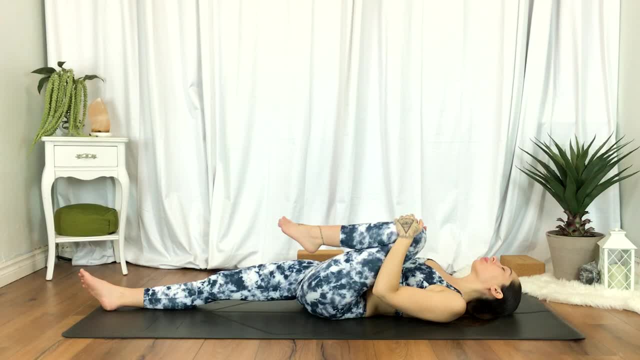 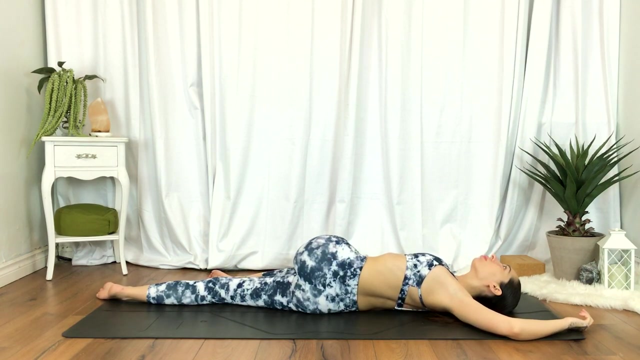 Exhaling, softening the belly, Observing what's happening here. The left side too Exhale. we'll cross the left knee over towards your right Option to modify: Listening to the body and softening the belly with each exhale. 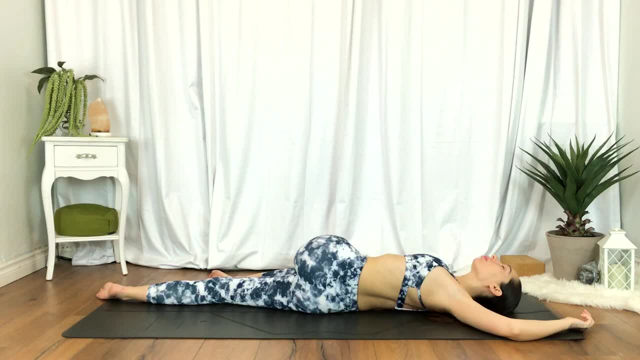 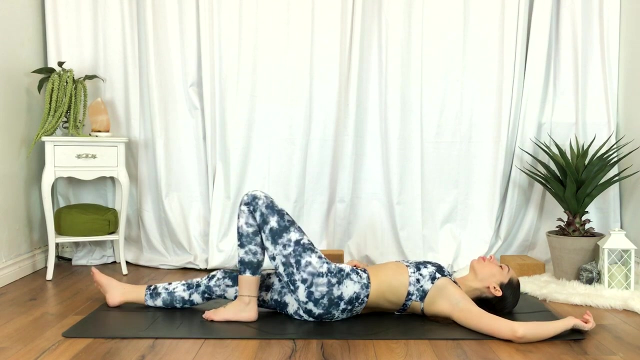 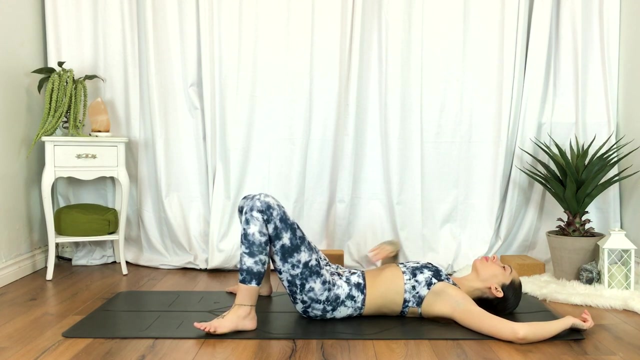 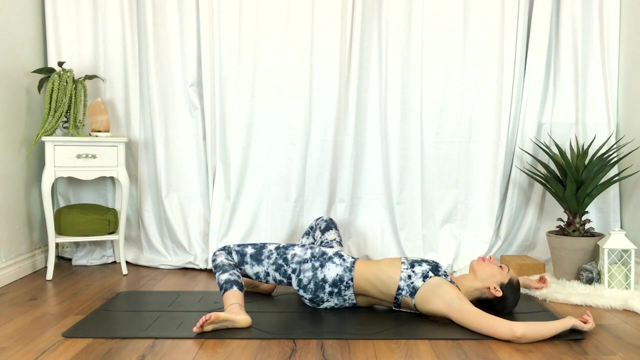 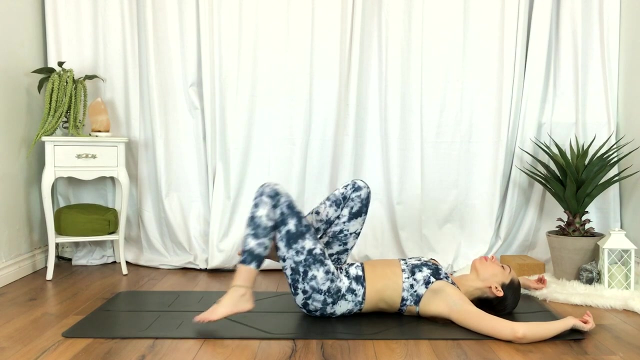 Inhalation, Exhaling. Thank you, Thank you, Thank you. Inhale release: Gently rocking the knees side to side, Elbows in line with the shoulders. Inhale release: We'll go ahead and hug both knees towards the chest. 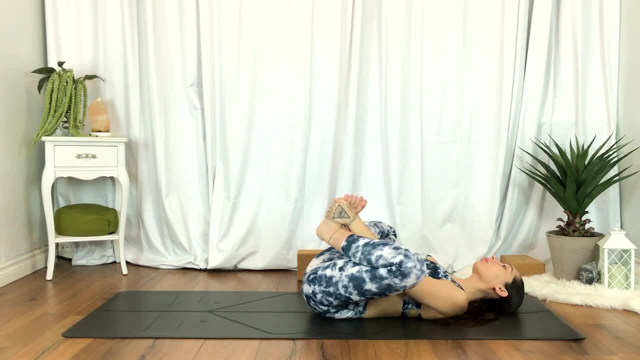 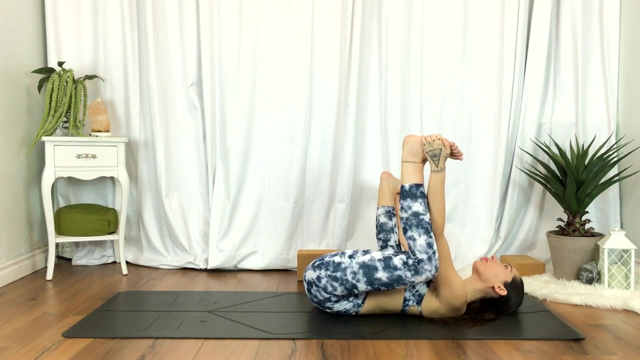 Grabbing the outer edges of the feet Resting right here or open the feet for happy baby pose. Option to rock side to side. Inhale release- Exhale release. Exhale release- Inhale release. 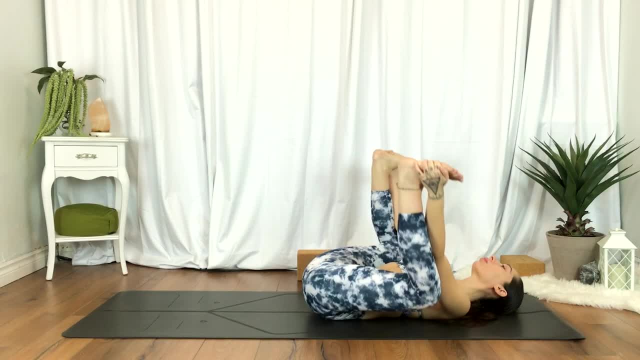 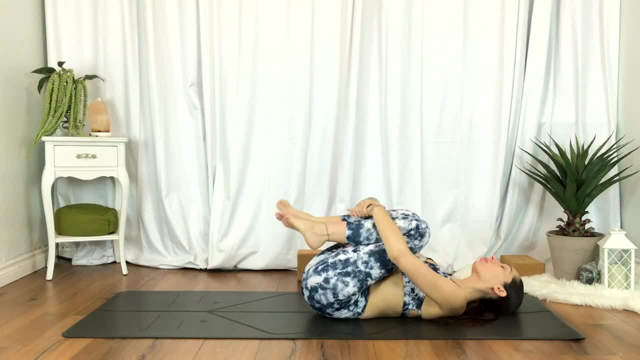 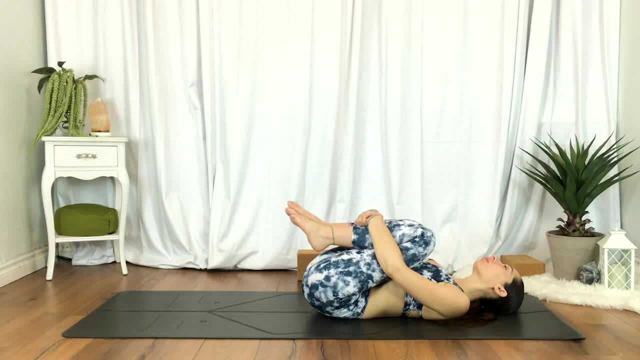 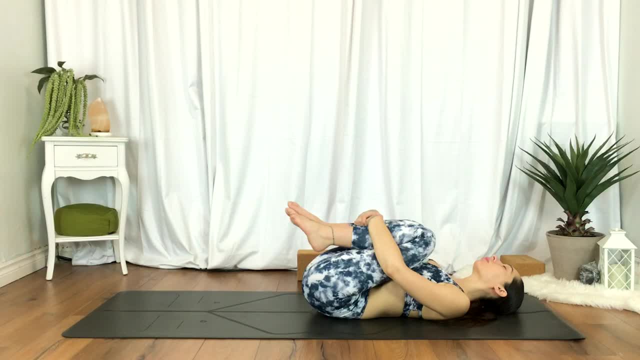 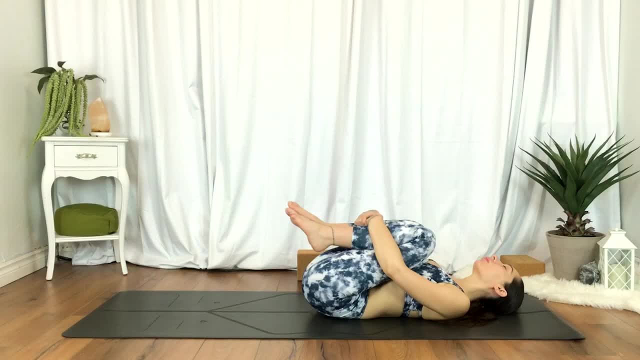 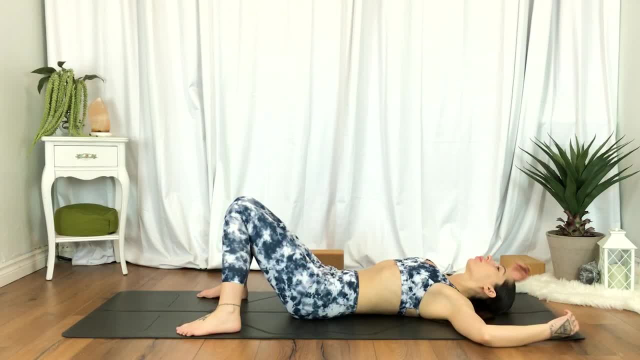 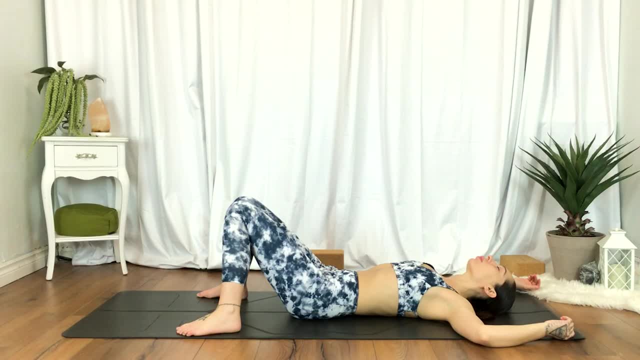 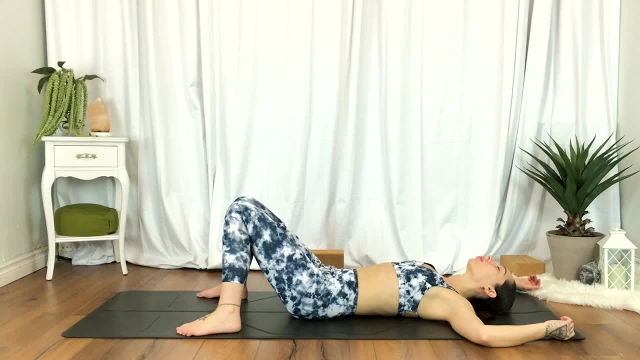 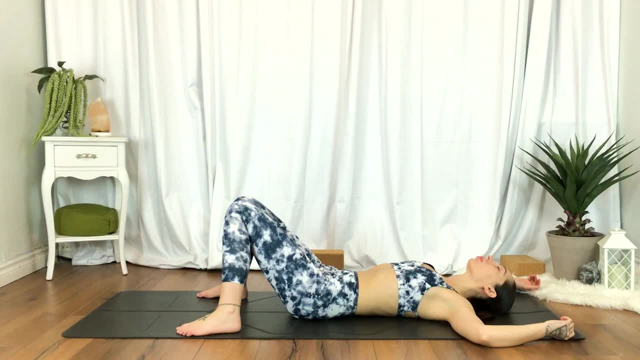 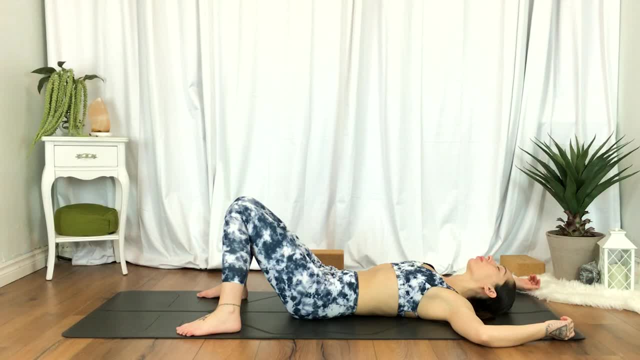 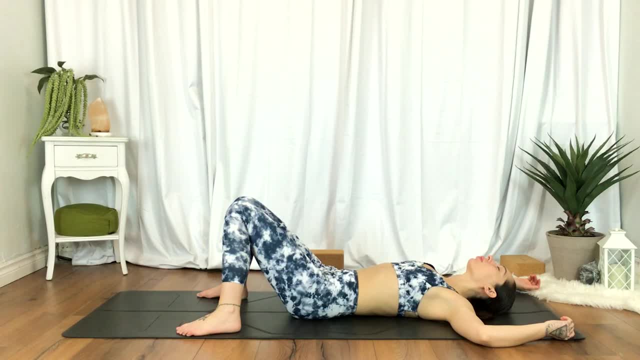 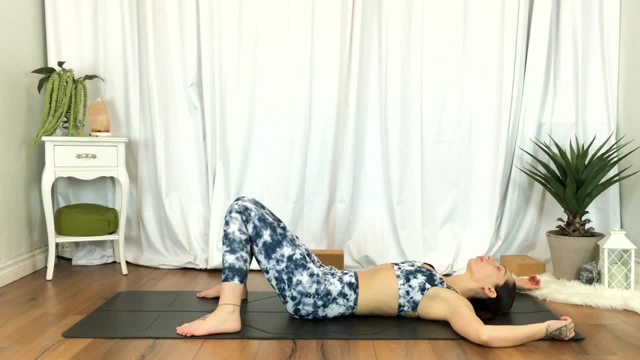 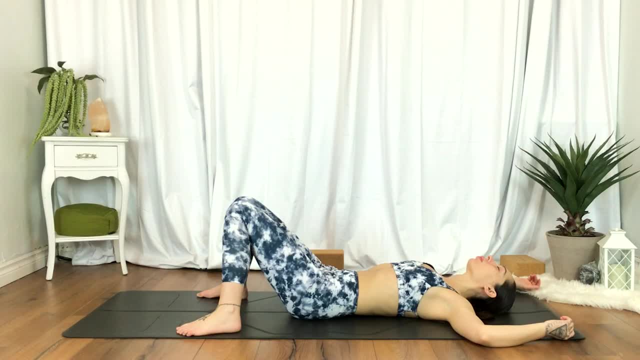 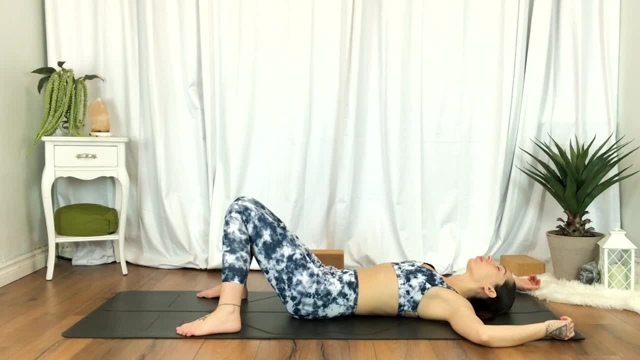 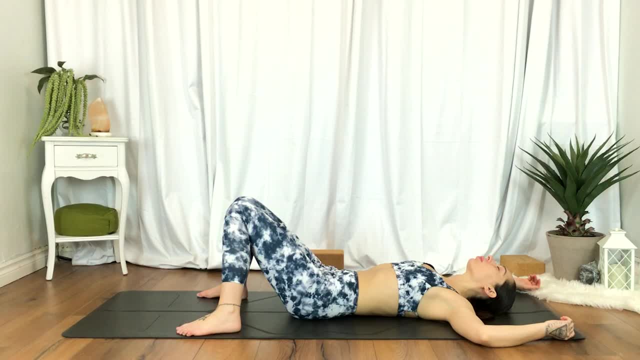 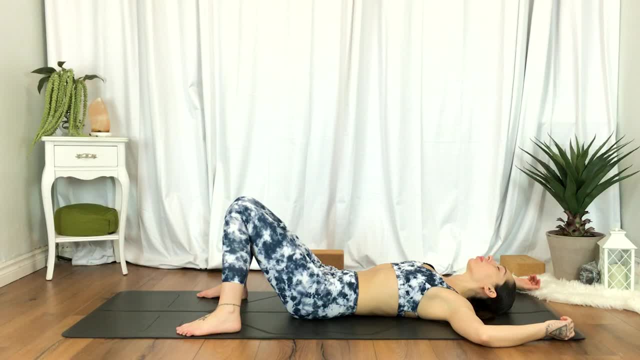 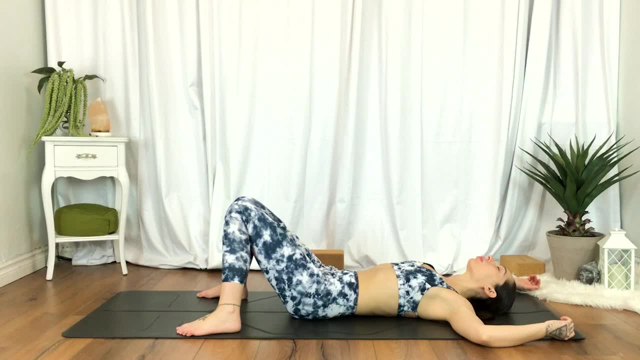 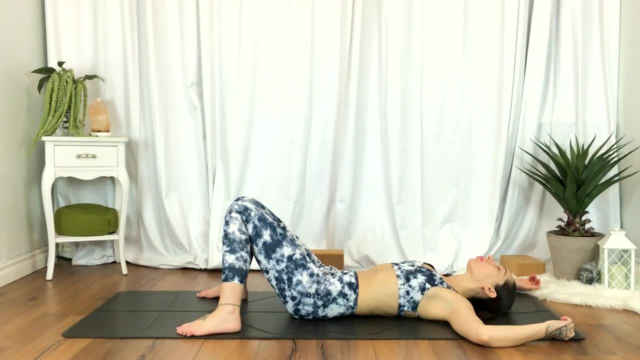 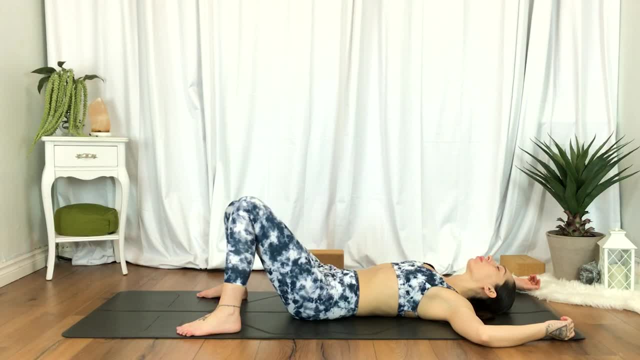 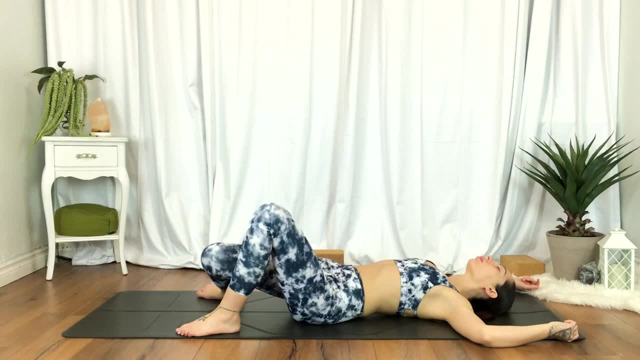 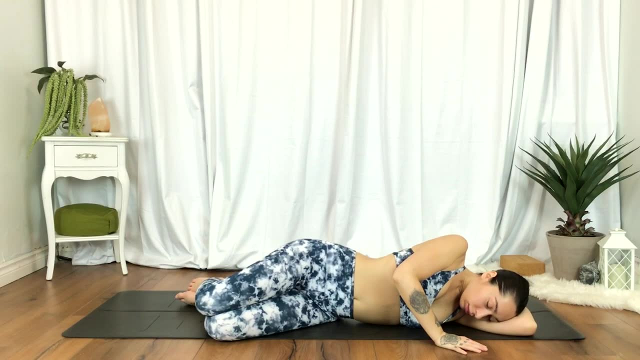 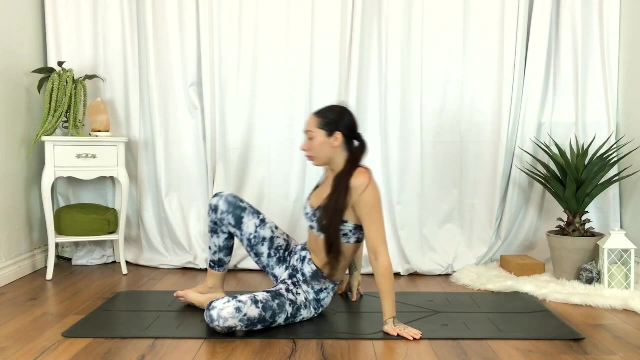 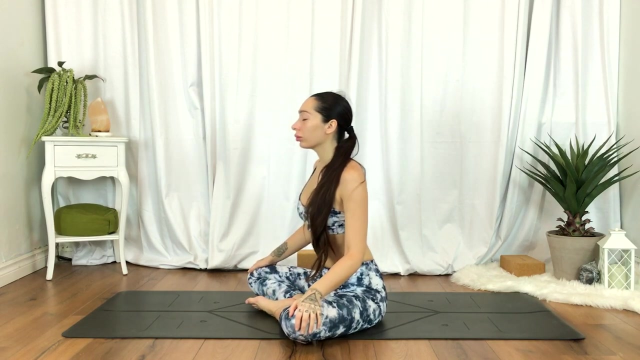 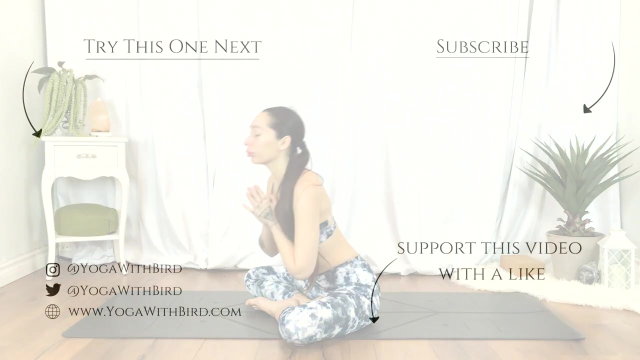 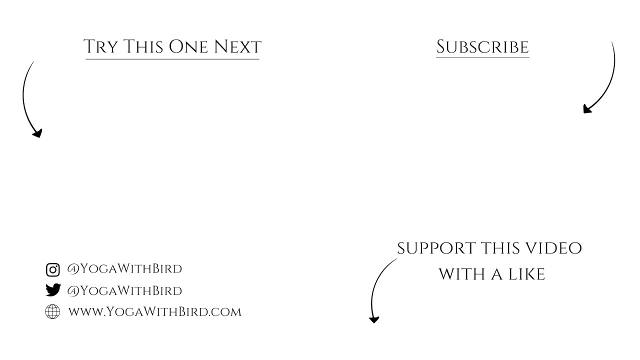 When you're ready, we'll roll over towards the right. Full inhale and exhale Gently. come to seated. Inhale hands up overhead, Inhale heart center. Thank you for joining Namaste. If you enjoyed this video, don't forget to like it below. subscribe to my channel and. 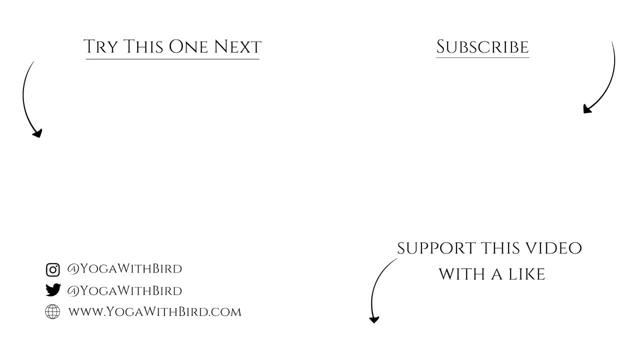 hit the bell icon so you don't miss any updates on future videos and live streams.